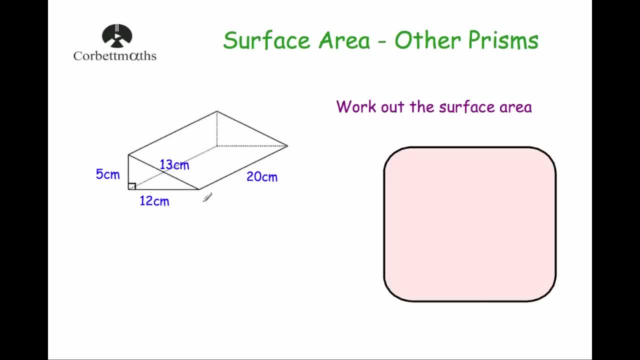 a height of 5 and a hypotenuse of 13 and the length of the prism is 20 centimetres and the question says: work out the surface area. So the triangular prism has five faces. It's got the triangle at the front, the triangle at the back, it has got the rectangle on the bottom, it has the 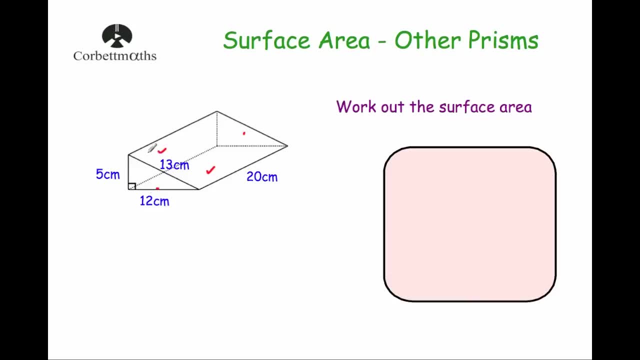 rectangle, which is the vertical one on the left hand side, and it has got the sloped rectangle as well. So it's got five faces. I've got the net here, if it helps to sort of show where it's got the bottom, the sloped face, the two triangles and the vertical side and they would all fold up to. 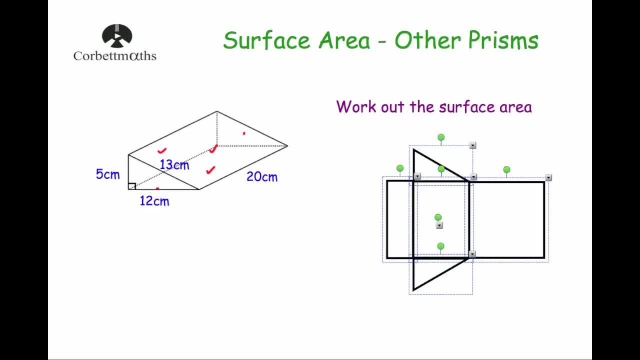 make that triangular prism. So let's get started. So let's call the two triangles 1 and 2, the base of it. let's call that face 3, the vertical rectangle 4 and the sloped one 5.. Okay, so triangle 1 and 2.. So there, if a 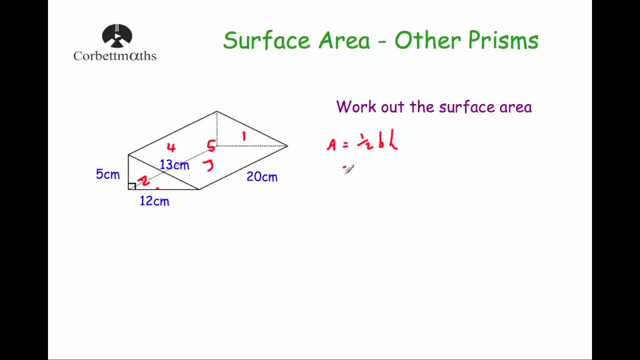 triangle is equal to half the base times the height. So the base of the triangle is 12, so half times 12 and the height of the triangle is 5.. So we're going to do half of 12, which is 6 times 5. 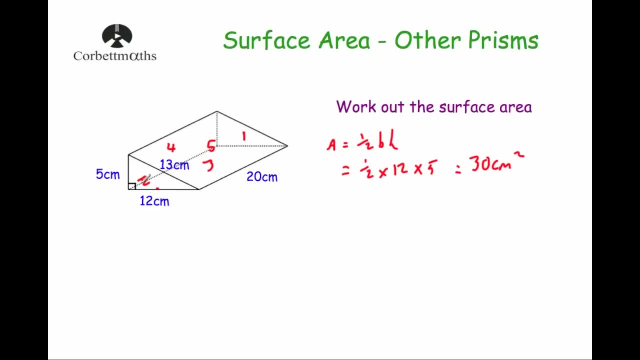 is 13.. So we're going to do half of 12, which is 6 times 5, is 13.. So we're going to do: half of 12 times 6 is 15, and we put 6 on top of 5, which is Angle 6. so we've got the top of 12 and we're. 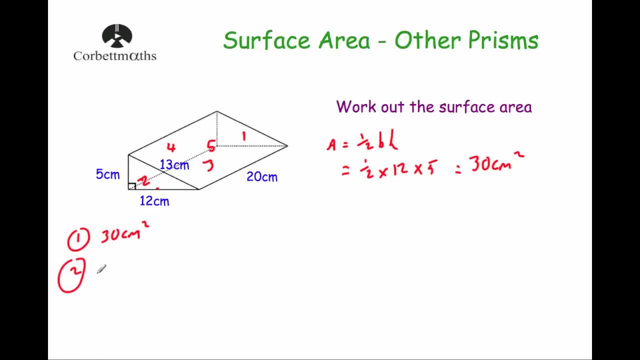 going to do the bottom 1. Reduce both sides by 3, because we don't want to have one encourage the other side of a circle. so there's only thirty 9 in the right side Right, so it's 30 cm°, and 1 is 30cm squared, So that's the area for the triangle at the front and the triangle at. 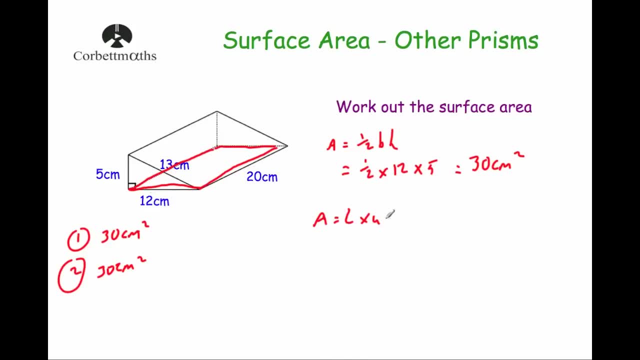 the back. So one is 30 cm² and 2 is 30cm squared, which is 20, times width, which is 12, which equals 240 centimetres squared. So that means face number three. the base has an area of 240 centimetres squared, So we've done three of the 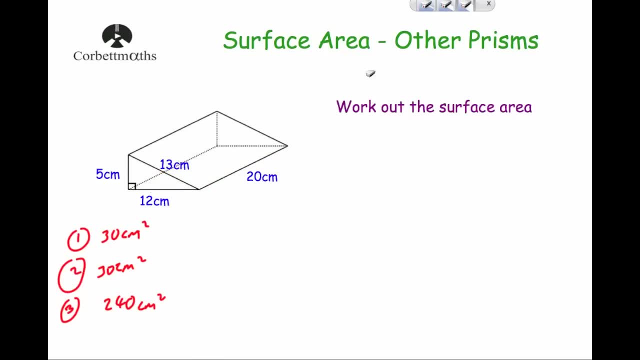 faces. We've done the triangle at the front, the triangle at the back and we've done the base. Now we're going to do the rectangle which is the vertical one on the left-hand side, this rectangle here, So that rectangle, it has a length of 20 as well and it has got a width of 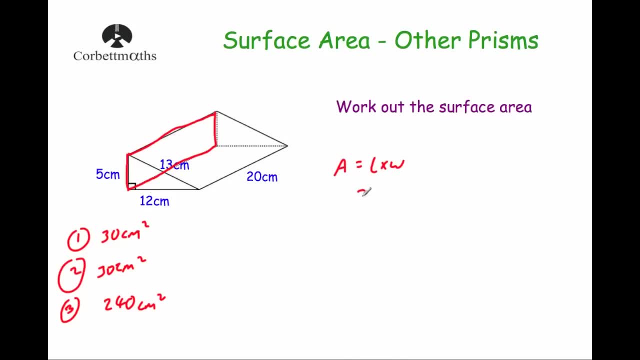 five. So area equals length times width, which would be equal to 20 times five, which would be equal to 100 centimetres squared. So that was face number four, the vertical one, which is equal to 100 centimetres squared, And finally we have got the rectangle, which is the sloped face. 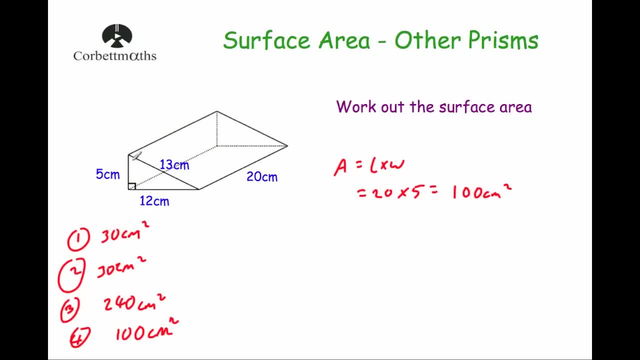 So that rectangle is this rectangle. here and again, the area is equal to length times width. So it's going to be the length which is 20, and the width, which is equal to 13, this time okay. So 20 times 13 is 260. 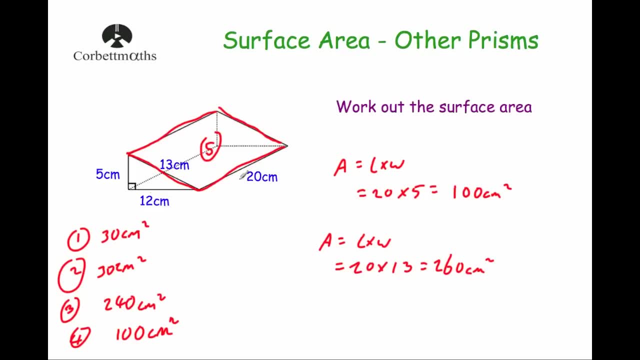 centimetres squared. So that was face number five, the sloped face, And then all we need to do is add those area of those five faces- the front, the back. so the front, the back, the bottom, the left. 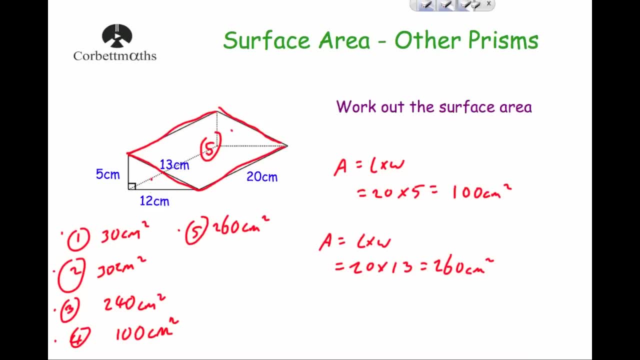 and the sloped one, And they will give us a total surface area of this shape. So the total surface area, total surface area will be equal to 30 plus 30 plus 240 plus 100 plus 260.. And when we do that we get. 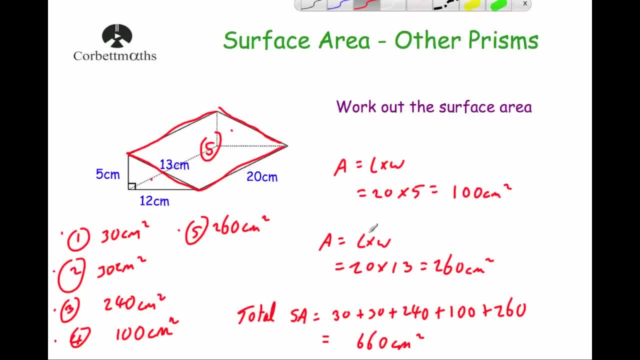 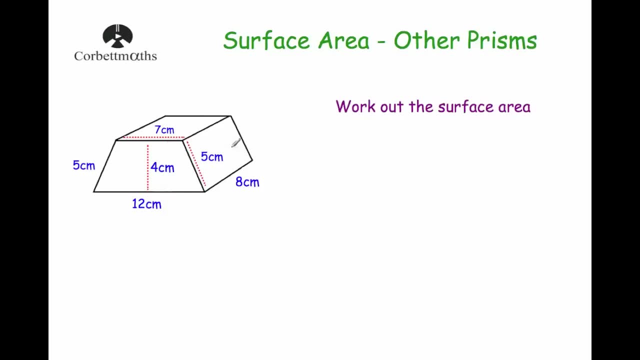 660 centimetres squared, and that's it. Okay, so we're now going to work out the surface area of this trapezoid prism. So, as you can see, it's got a trapezium at the front, it's got a rectangle on. 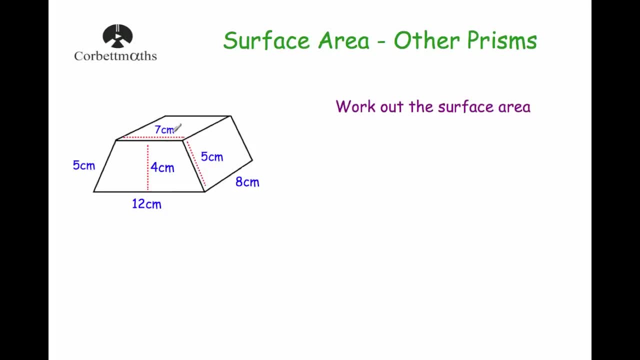 the right-hand side, a rectangle on the left-hand side and a rectangle on the left-hand side. So we're going to work out the area of those six faces and then add them together to get the total surface area of this trapezoid prism. Okay, so let's start off with the front, The area for 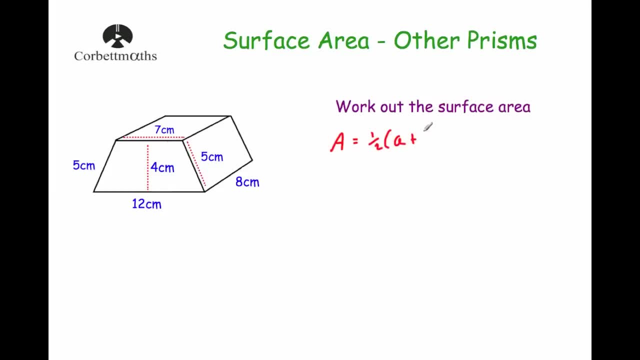 trapezium is equal to a half bracket a plus b times h, And if you can't remember that, watch the video on Corbett-Marvs on that. okay, Area for trapezium. So a and b are the two parallel sides. 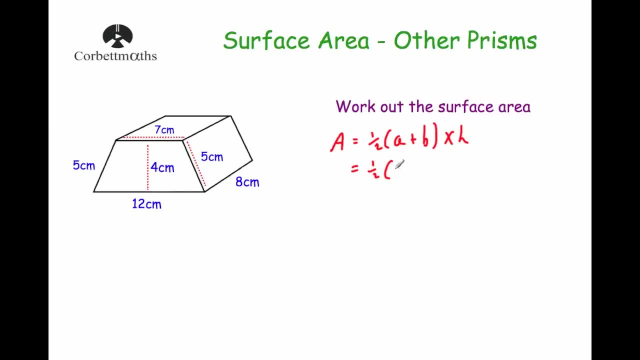 so that's the top and the bottom. So that's seven plus 12, and that's a half bracket a plus b times h, And then we're going to times that by the height of the trapezium, which is four Ignore. 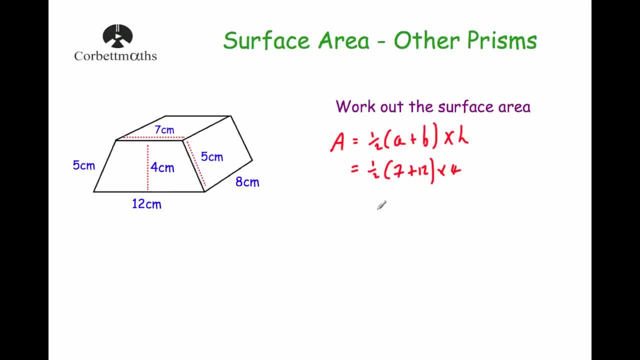 five. that's the diagonal, it wouldn't be the height. so four is the height of the trapezium, So seven plus 12, we're using BobMass to do the brackets first. seven plus 12 is 19, and half of. 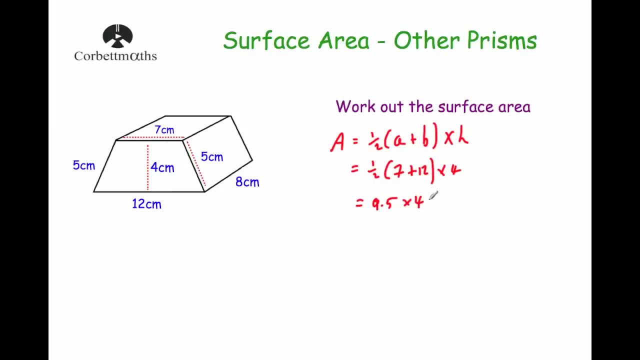 that is 9.5.. And then we're going to times that by four and that will be equal to 38 centimetres squared. So that's the area of the front which is going to be- let's call that one- the back. 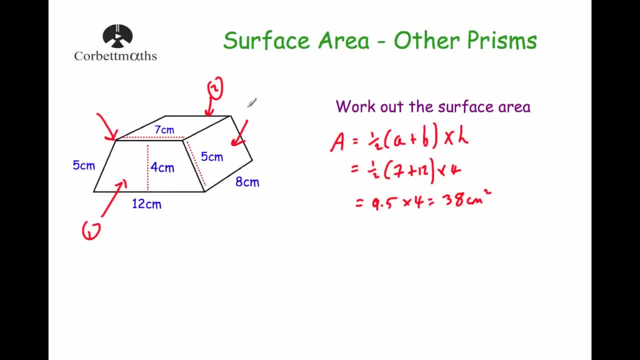 which is two, the left and the right, Which we'll call three and four, and we'll call the top five and the bottom six. So that is the area of one, the front, 38 centimetres squared, and it's also the area of the back. 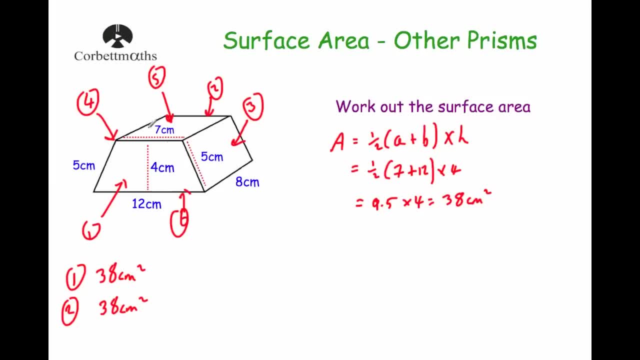 which is 38 centimetres squared also. Okay, now let's look at three and four, which are the two rectangles. Now, as you can see, the trapezium has got the length of the sort of the side of the trapezium on the left and the right are both five centimetres and the 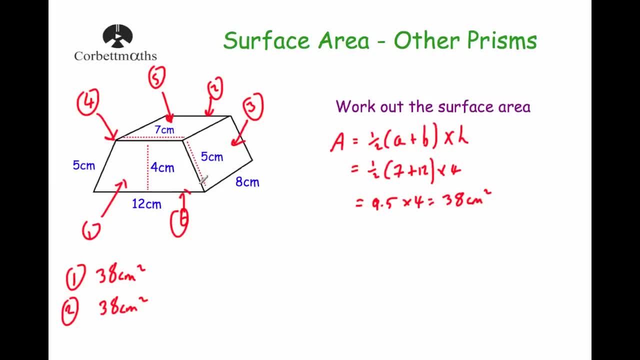 length of the trapezium is eight centimetres. So if we do, if we look at this rectangle, if we do eight times five, we're going to get the area of that rectangle. So area equals eight times five, or length times width, which 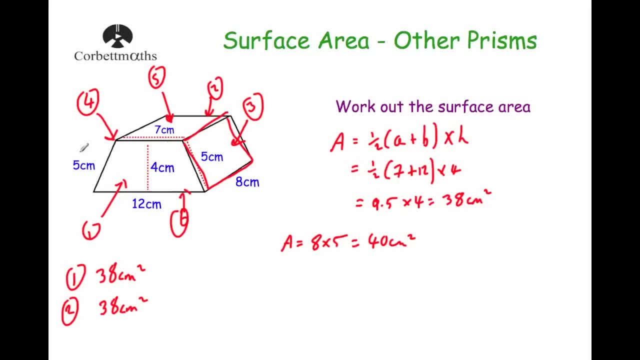 is equal to 40 centimetres squared, And that's the same for the left hand side also, because it's also going to be five times eight. So that means that the area of three is equal to 40 centimetres squared and the area of face four is also equal to 40 centimetres. 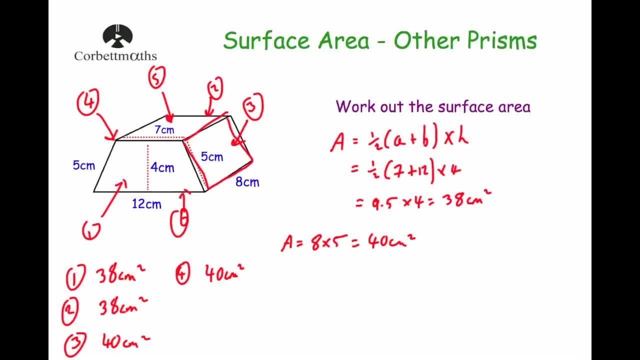 squared. Okay, face number five: Well, that's the top of the trapezoid prism. So if I just rub this out, we can have a look at that. So the top is also a rectangle And if we look at it it is seven wide and it is eight long. So we're going to do and. 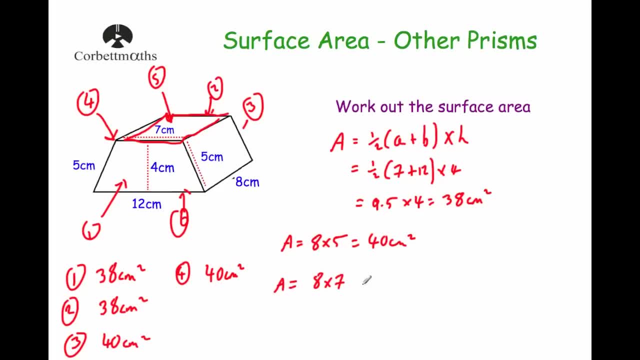 it's a rectangle. so area equals eight times seven, which is equal to 56 centimetres squared, because it's seven times eight. seven times eight is 56. And that's the area of the top. that's 56 centimetres squared. And now just the bottom. So the bottom also is a rectangle. 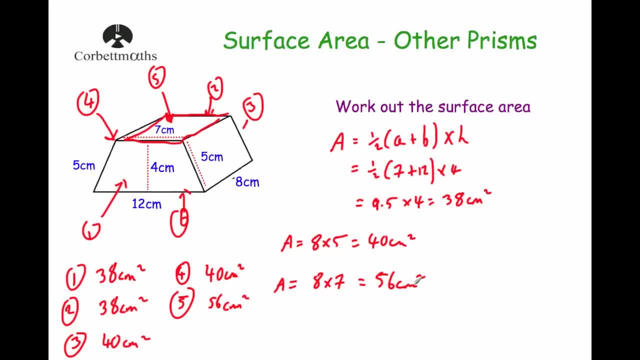 and it's going to be 20 centimetres. So that's the bottom, And then the top is going to be 12 wide and eight long. So we're going to do: area is equal to 12 times eight, which is equal to 96 centimetres squared.